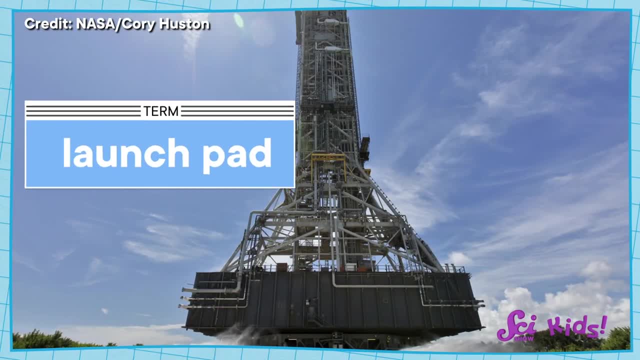 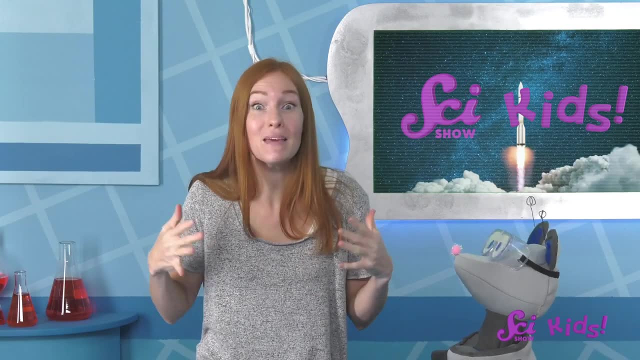 That's what all of the fire and smoke is. Beneath the rocket is the launch pad. It's made of concrete and is super strong. When it's time for launch the rocket engines mix and heat up two things called hydrogen and oxygen. 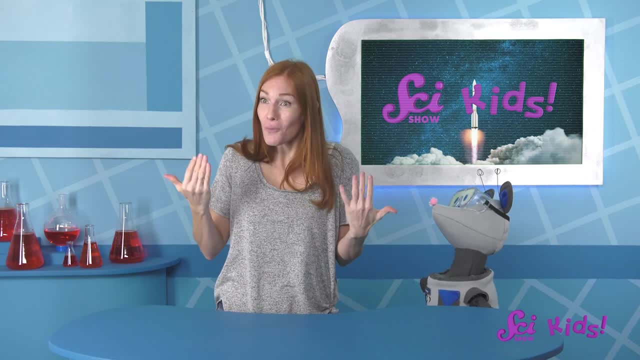 They're both all around us in the air all the time, Even though we can't see them. Ooh, good thinking Squeaks. We do use oxygen in a special way. We breathe it, But when oxygen and hydrogen mix together and they get really hot, they combine and 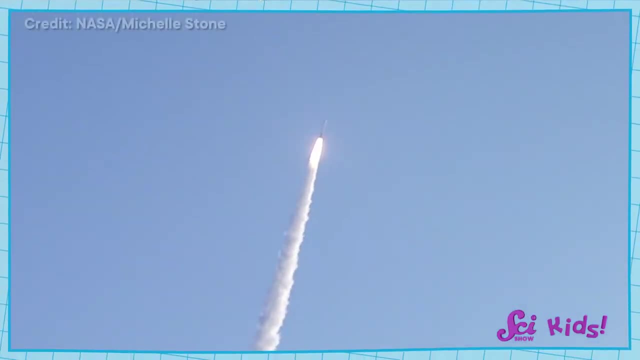 form this really huge cloud that rushes out the end of the engine super fast And it pushes against the launch pad hard, Really hard. Do you remember what we call something that pushes or pulls A force? You're right. This huge push is a huge force. 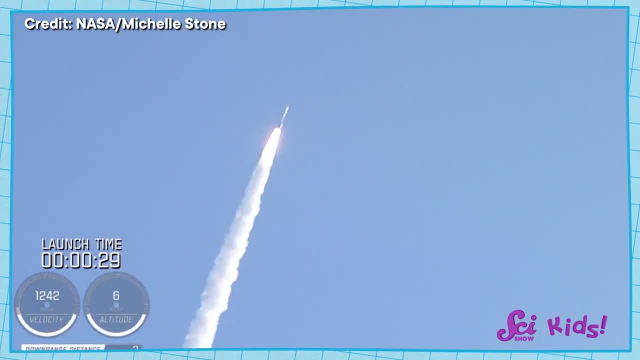 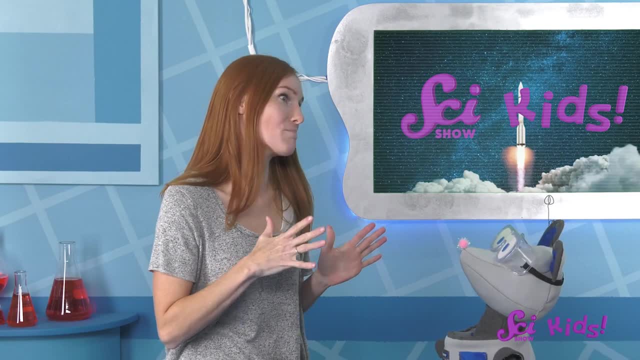 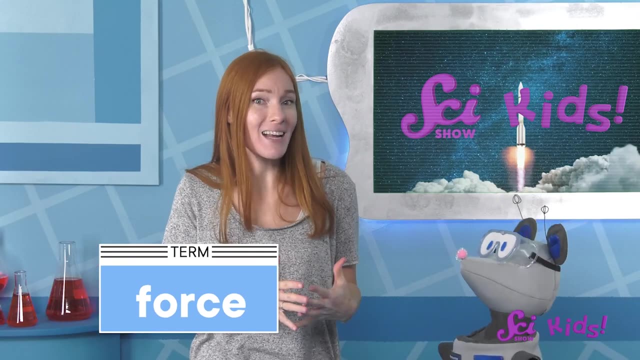 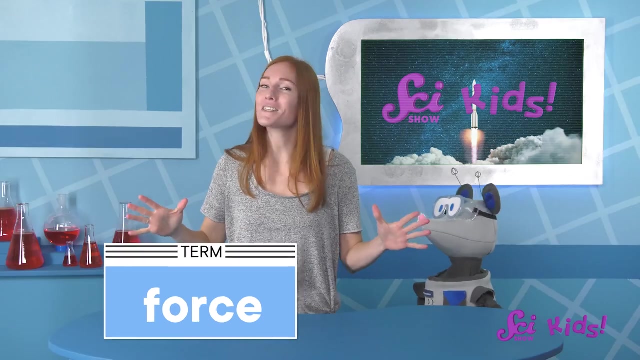 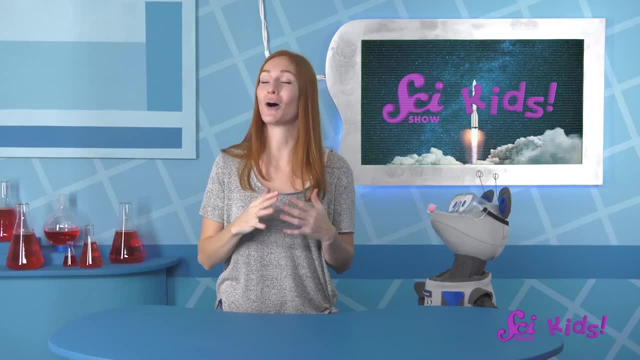 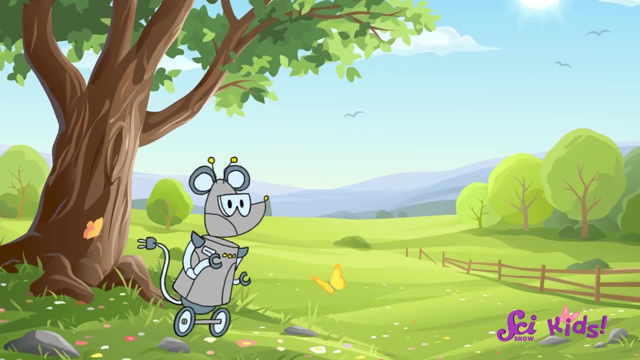 Forces are all around us and we see and feel their effects all the time. For example, a force called gravity keeps you, me and everything around us on the ground. If gravity didn't exist, there'd be nothing to keep us on the ground. 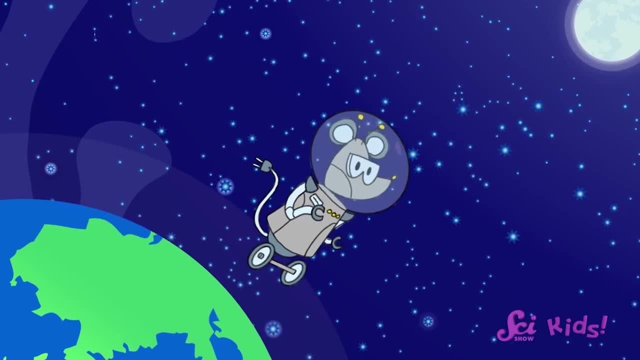 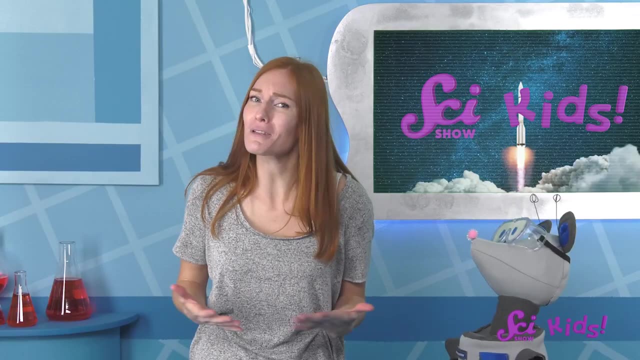 So even a tiny hop could send us off into space. So thankfully, Earth's gravity is always pulling us. Oh, that's fair enough. We usually don't feel like we're being pulled on by the force of gravity, But that's just because we're used to it. 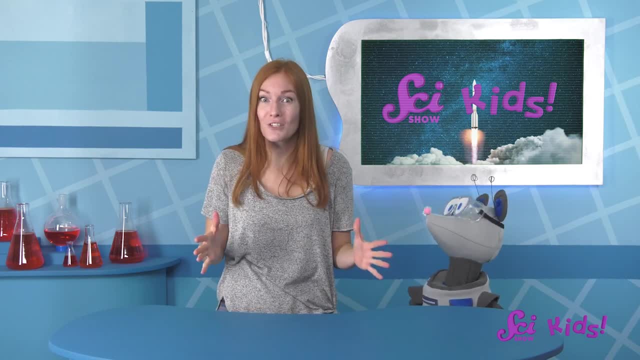 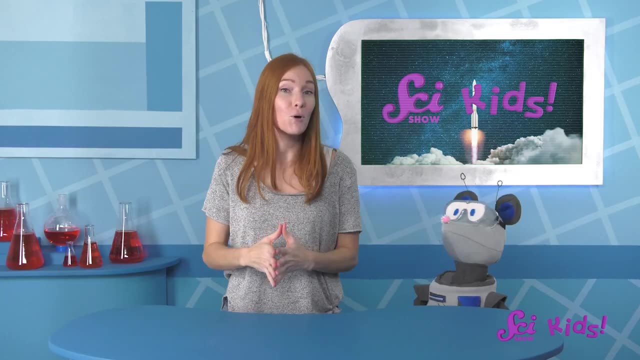 And there's a simple way to feel the force of gravity: All we have to do is jump Ready, Jump. When we jump, we make a force because we're pushing down on the ground with our feet And that makes us go up. 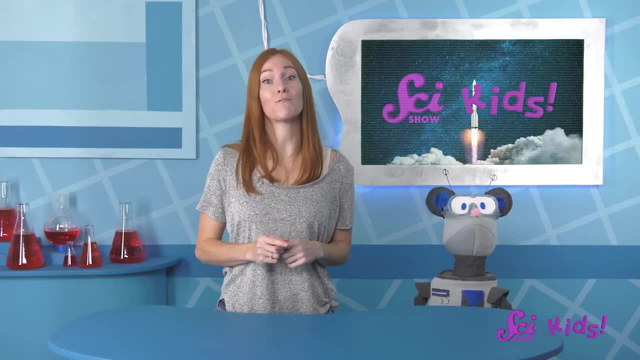 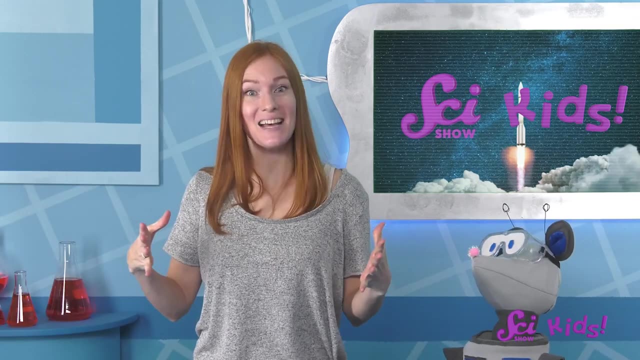 But we didn't keep going up, did we? That's because once our feet left the ground, gravity took over and pulled us back to Earth. A rocket is basically the same idea as us jumping into the air, but on a much bigger scale.